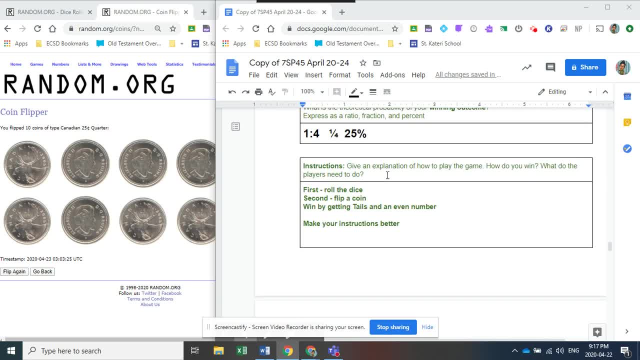 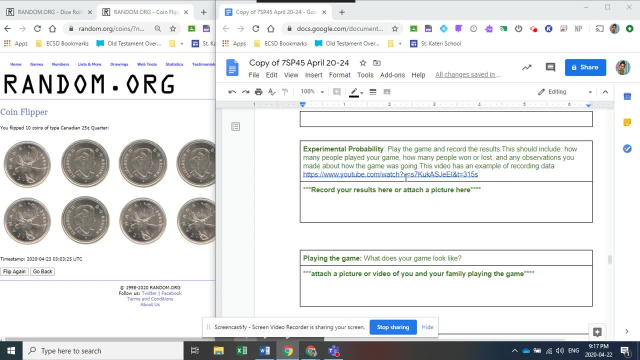 All right. so we just finished the theoretical probability of this game, and now we're going to go on to the experimental probability. Make sure you watch this video too, if you want to see another example of how to make experimental probability. Right here is where you're going to record your results. Either you can tally it on your 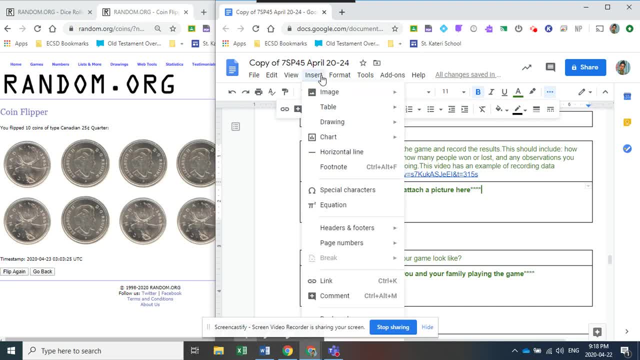 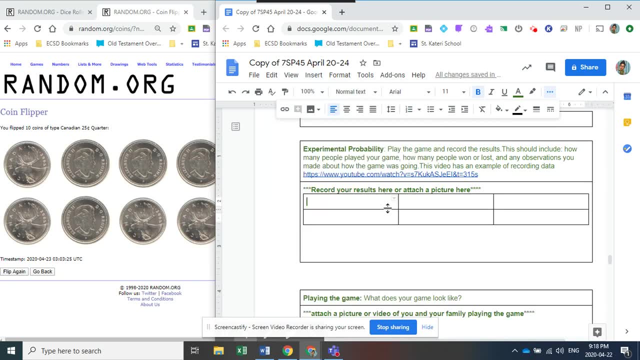 own, or you can like attach a picture or just put a table right in here. I'm going to put the table right in here, So I'm going to put on this table. I need one more row. you get tails and even number. Okay, so that's how I win, And not tails. 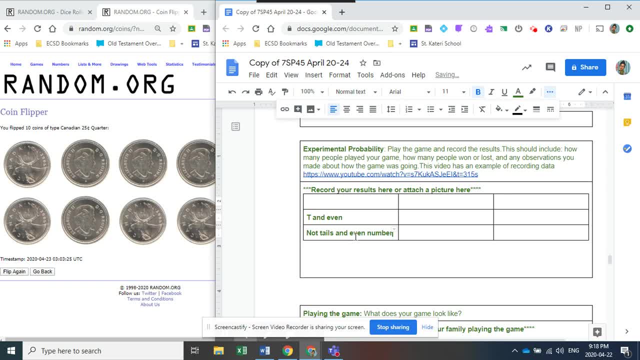 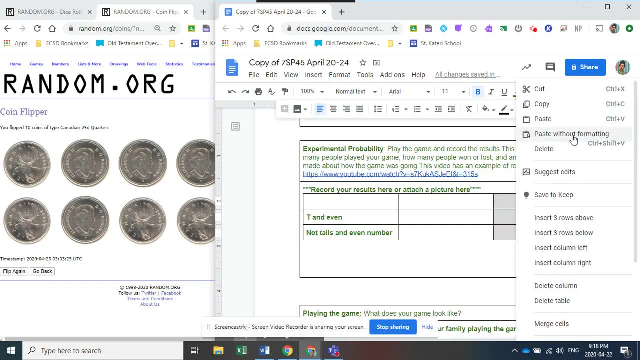 And even number Three years looks better than mine, see. And then on the top, I'm just going to write down how many trials I do. So let me get rid of this row too. I don't want this Delete. 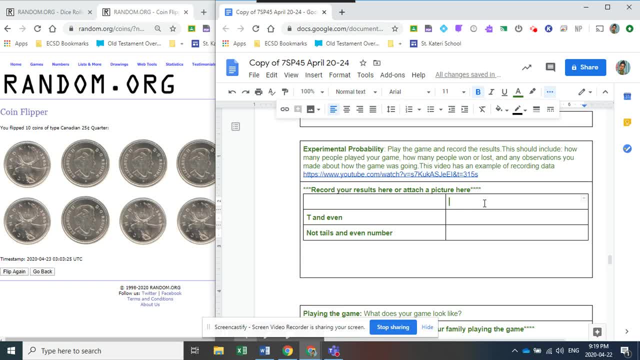 call All right, so I'm going to do 10 trials or play 10 times, So that's 10 games or whatever. All right, so that you could see this. I got this. I went on randomorg and it has a bunch. 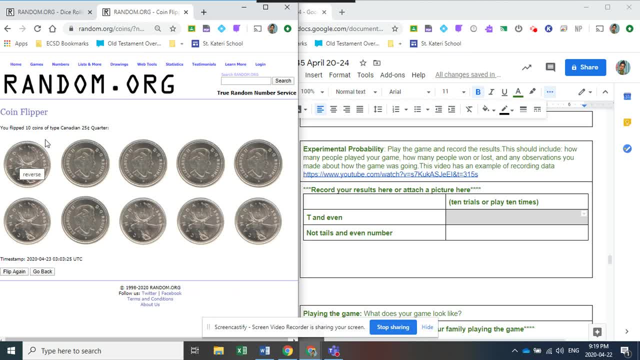 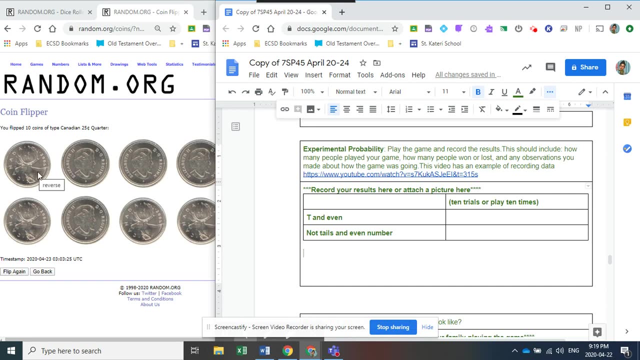 of randomizers, And so this site randomly flipped the coin 10 times for me, And so I'm just going to record on here all the outcomes. So I'm going to put that under here, and I do want you to include the outcomes so that I- I don't know- get more information. I'm going to put tails, heads, heads. 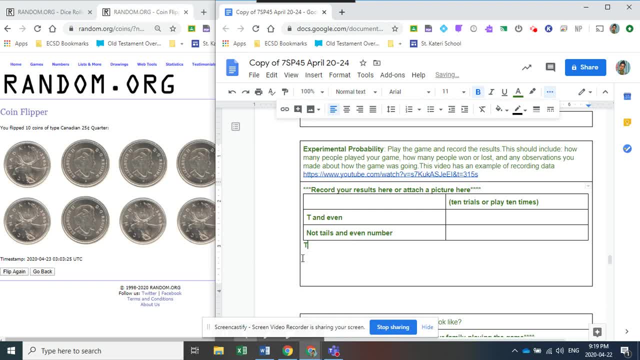 heads. Now, ideally you would flip a coin and then roll the dice, But because I can't really show you that and show you my screen at the same time, we're going to do them kind of super independently. Okay. so one, two, three, four, That's that one, And then on the bottom we have tails heads. 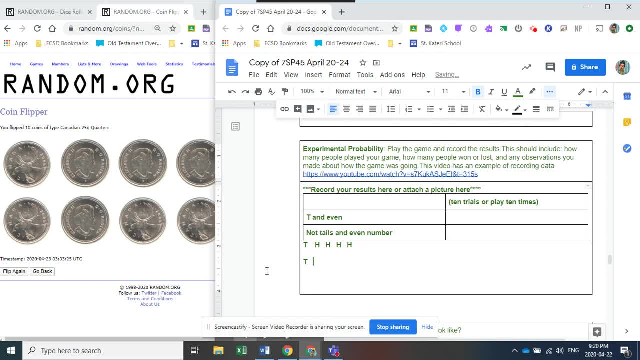 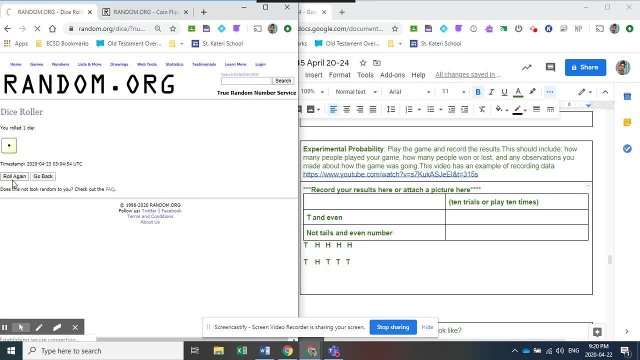 tails, tails, tails, Tails, heads, tails, Tails, Oops, Tails. Okay, so I have my 10 coin flipping there And I'm going to roll my dice 10 times. I got. well, I can start again, I guess. 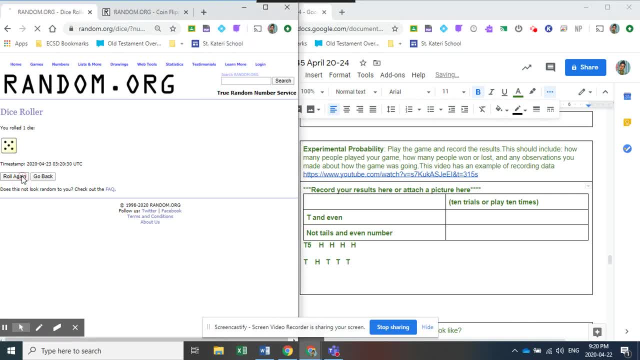 Roll the dice. I got a five. I got a two. Wow, this is very slow. 1,, 2,, 3,, 5,, 1, I think I got one again. 4,, 5,, 6,, 7,, 8,, 9,, 10,, 11,, 12,, 13,, 14,, 15,, 16,, 17,. 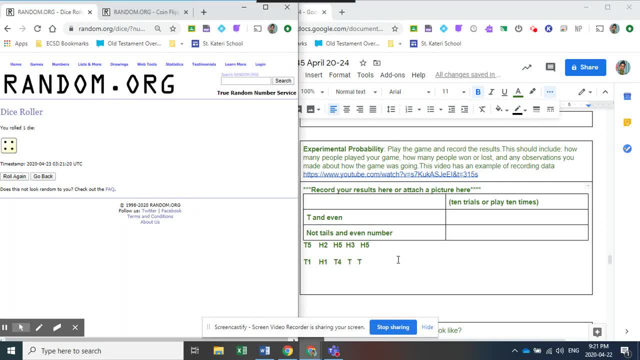 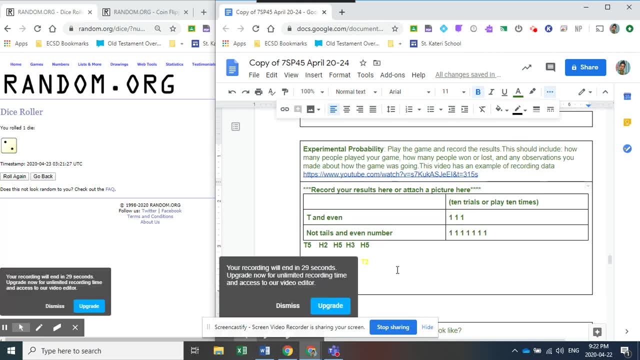 then I record my theoretical probability- sorry, my experimental probability here- and so I'm going to go 3 out of 10 times. I won as a ratio, 3 out of 10 times and 30%. all right, I'm running out of time on this video, but you can see that the theoretical was 25%. 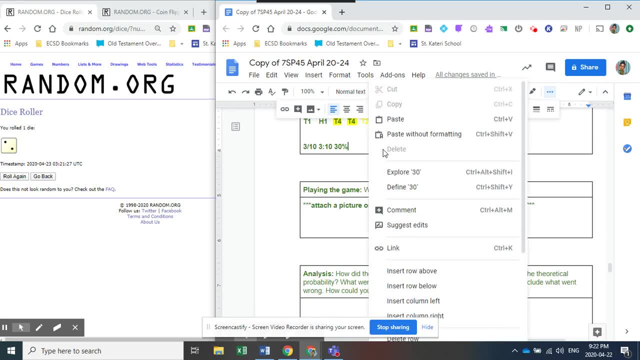 And you see that the experimental was 30%.